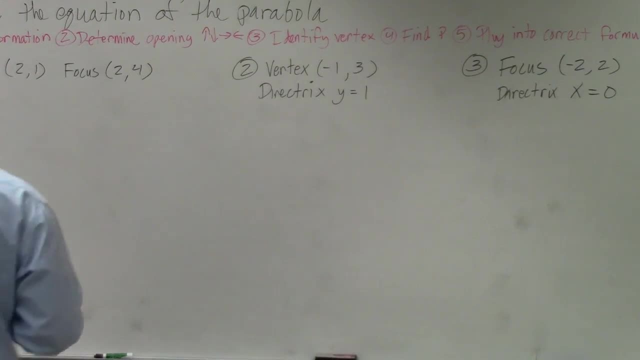 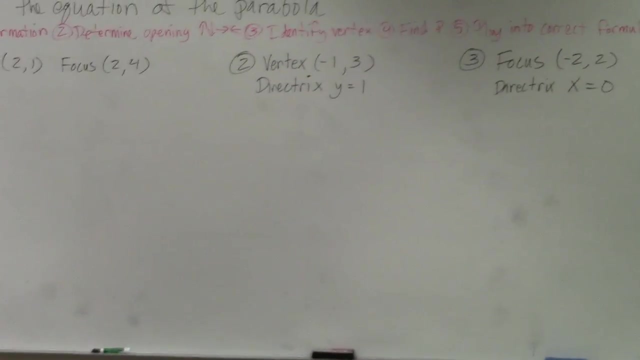 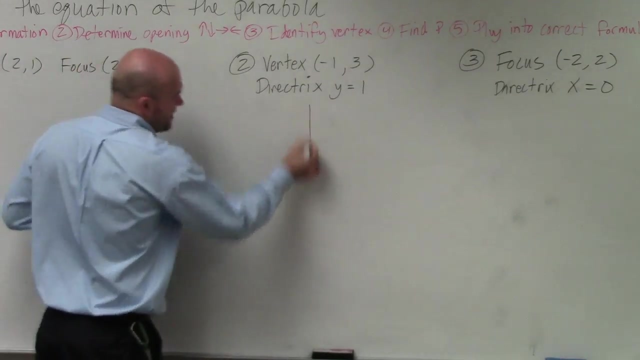 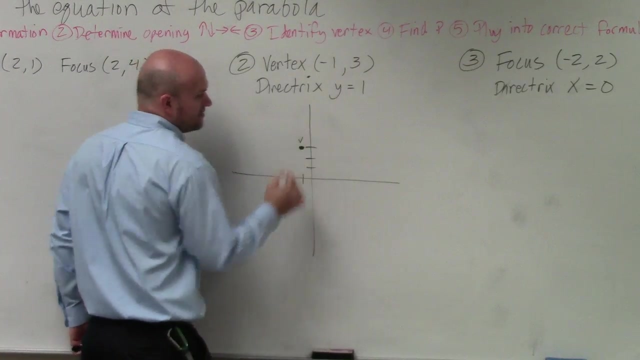 All right. so in this example- question number two again- if you guys remember, what I asked you guys to do was just to plot the information. So when you're trying to write the equation, the best thing to do is to plot the information. so therefore, you guys have an understanding of what you're looking at. So if you're going to graph it, you should graph it on an x and y axis. Vertex is negative, 1, 3.. And not only graphing it, but label it right, Because remember what happened when you guys were doing all this stuff? You guys had that initial point and all those red dots, right? 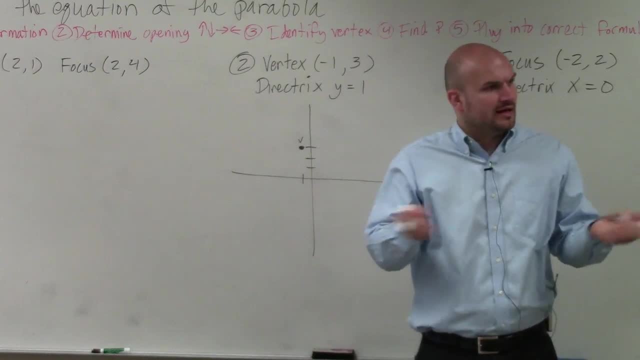 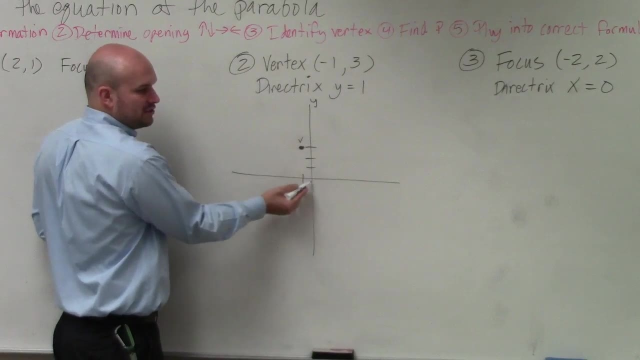 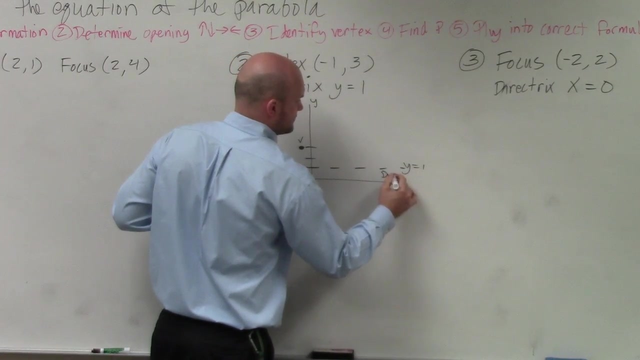 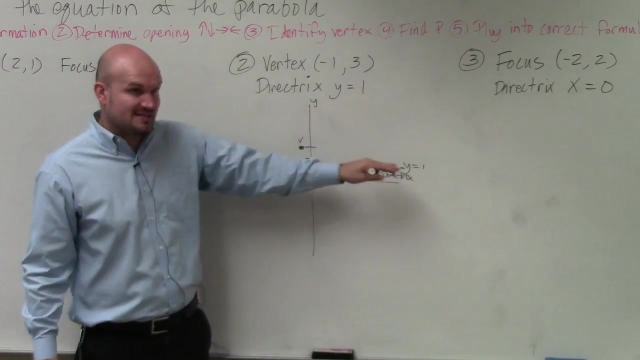 And one of the more common things I asked was: like: where's your initial dot? right, So label things. Hey, that's my vertex. The directrix is: y equals 1.. Well, here's the y axis. so when y is equal to 1, that's right there. So therefore, that's a horizontal line. That's my directrix. okay, Now we know. if here's my directrix, that's horizontal negative 1, 3.. Okay, so therefore we know that. 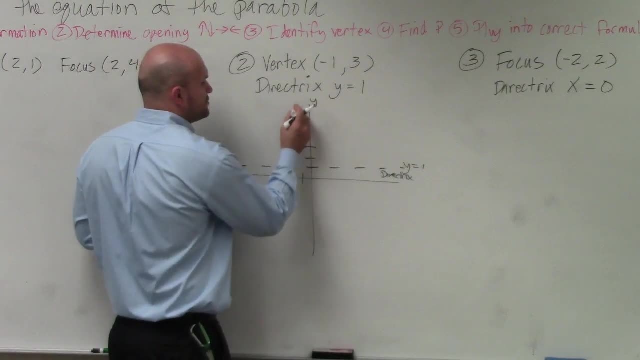 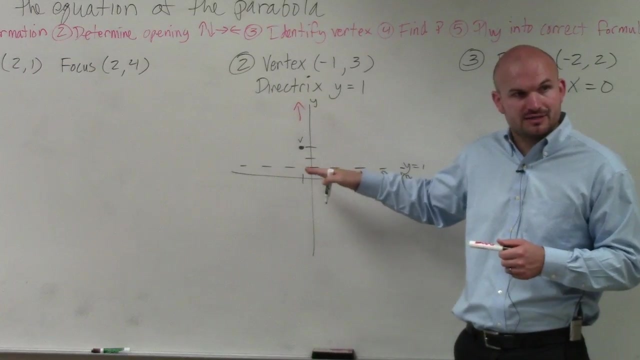 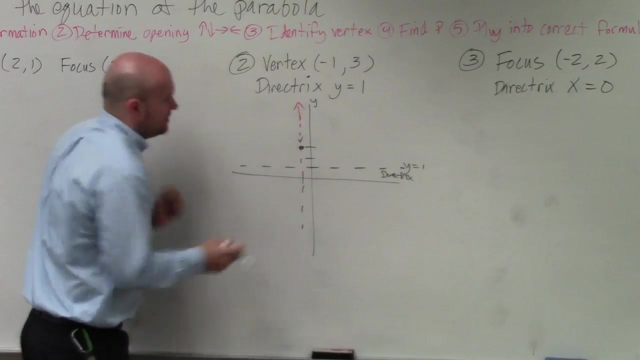 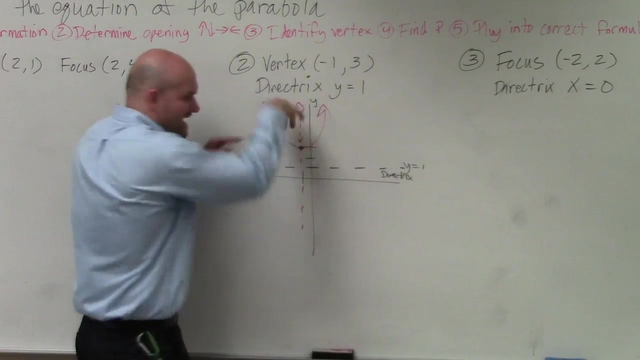 the focus. the graph has to open up towards my focus, right? It has to open up because it has to go away from the directrix Because, remember, the line of the axis of symmetry- Axis of symmetry- goes through your vertex and therefore is perpendicular to your directrix. So my graph has to look something like this: It can't open down, right, Because then it would be going into the directrix. That doesn't make sense, correct? 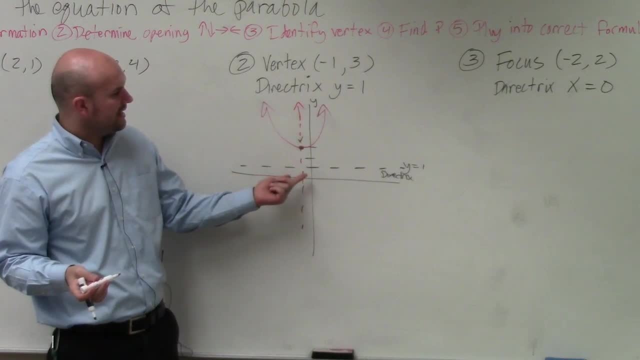 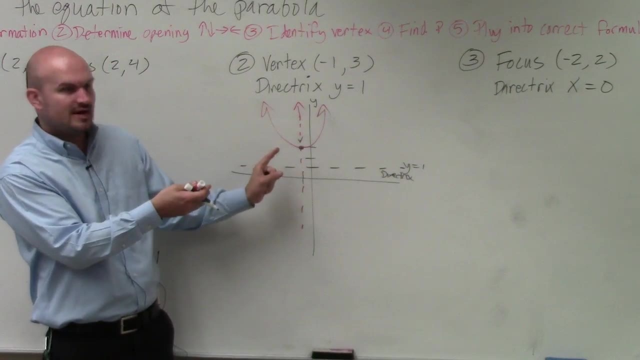 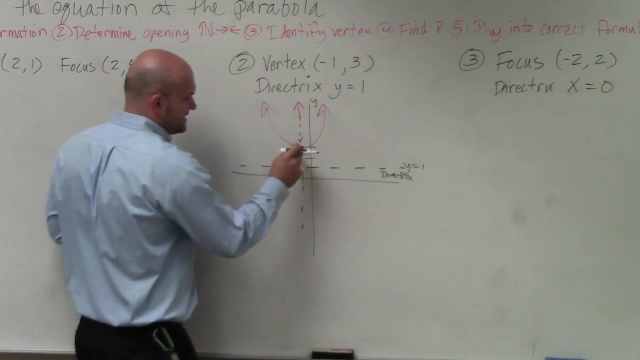 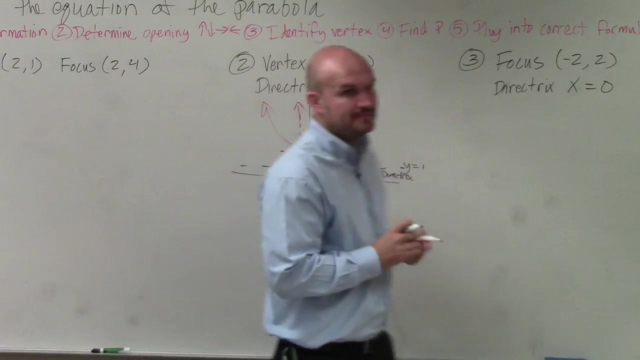 And the other problem is it can't open left or right, because then it'd be. you know, the directrix is perpendicular to the axis of symmetry, right, So that one makes sense. All right, so now we need to identify what the value of p is. Now we look at this distance between the vertex and the directrix, and that distance is 1,, 2, right, But the distance from v to the directrix, you're actually going where?